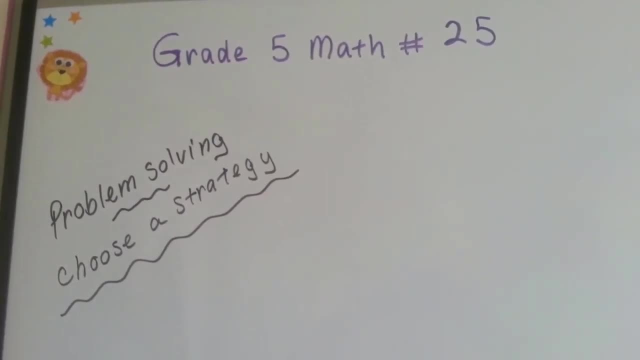 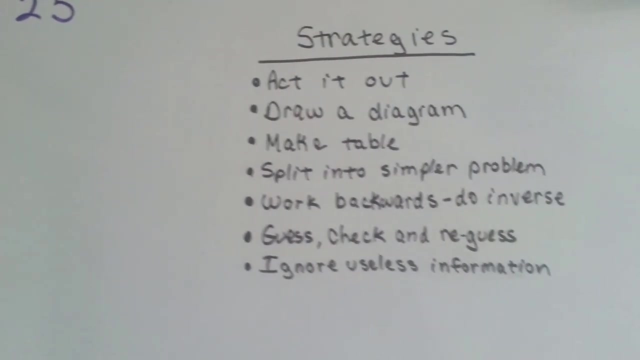 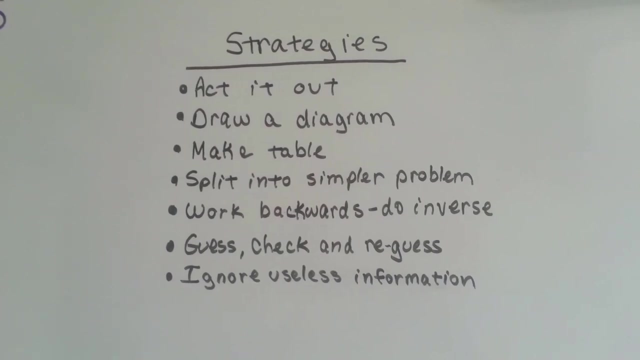 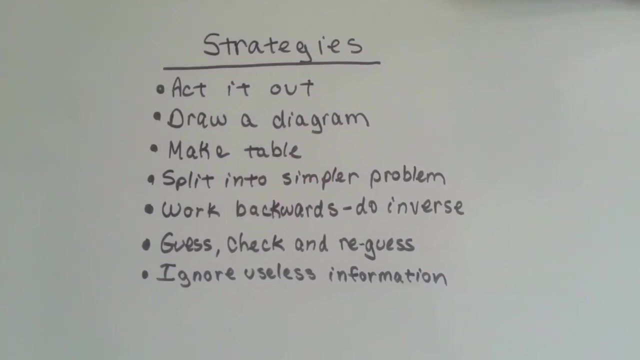 Grade 5, Math, number 25.. Problem solving: choose a strategy Now. we've done this before, but it doesn't hurt to keep trying them right. That way you really learn them. So here's our strategies. We can act it out, we can draw a diagram, we can make a table or a chart, we can split it into simpler problems, we can work backwards to do the inverse, we can guess and check and re-guess and we can ignore useless information. okay, 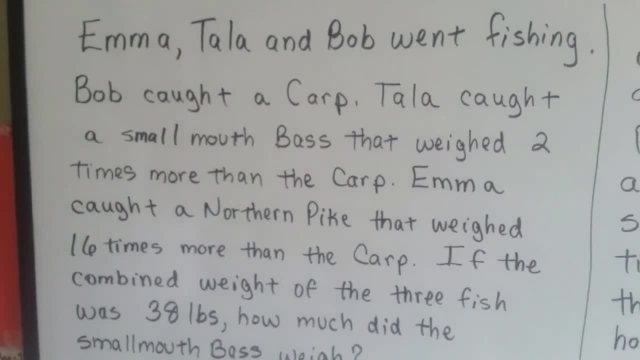 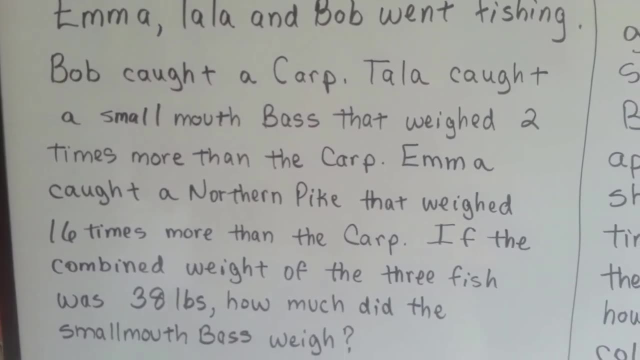 So here's our first problem. Emma, Tala and Bob went fishing. Bob caught a carp, Tala caught a smallmouth bass that weighed two times more than the carp, and Emma caught a northern pike that weighed 16 times more than the carp. 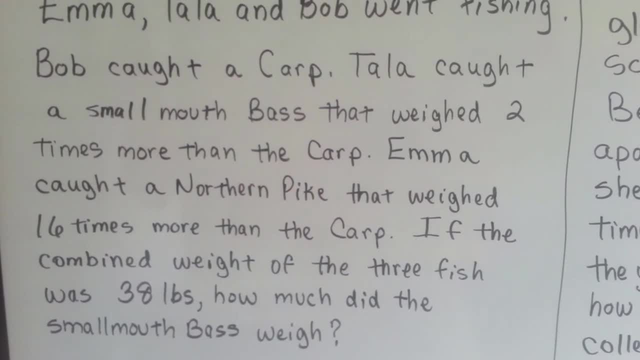 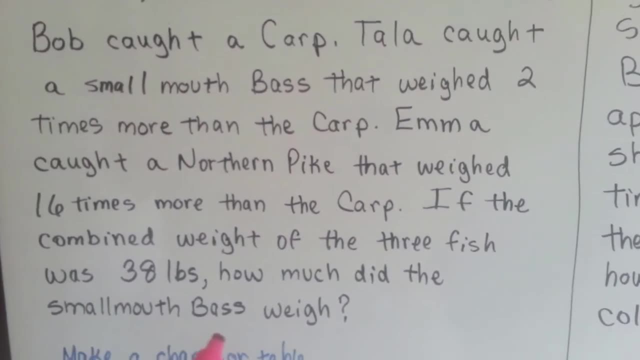 If the combined weight of the three fish was 38 pounds, how much did the smallmouth bass weigh? Alright, well, the first thing we've got to do is look at what it's asking. alright, It's asking us: how much did the smallmouth 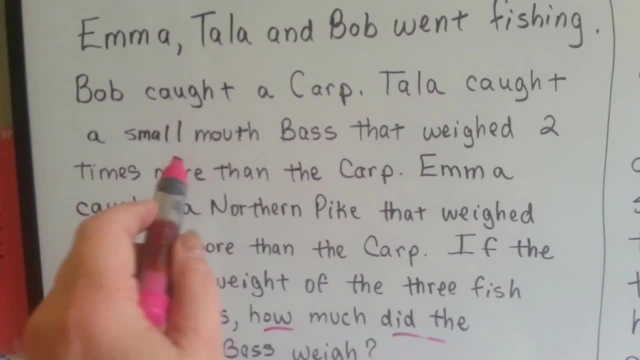 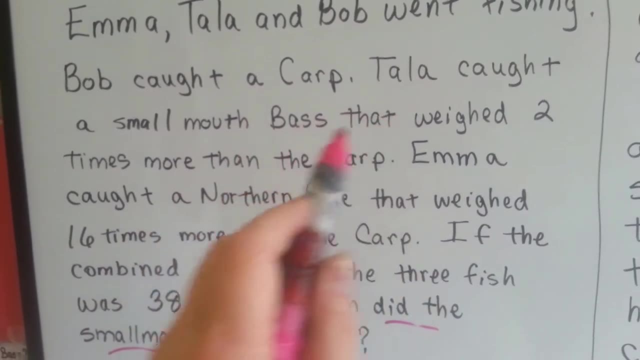 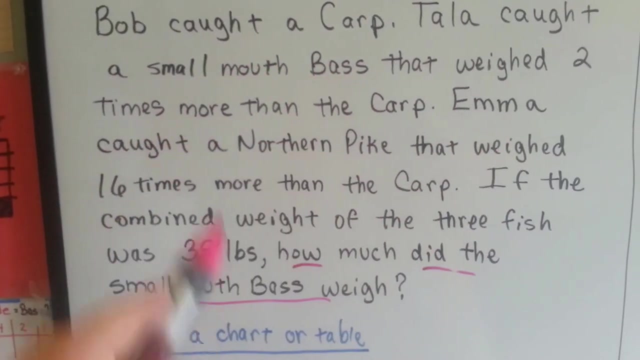 bass weigh. So let's go back and look. It was Tala who caught the smallmouth bass and it weighed two times more than the carp. okay, So we're looking for Tala's fish, alright. So I decided let's make a chart or table, because we've got so much information. the table will help us figure it all out, alright. 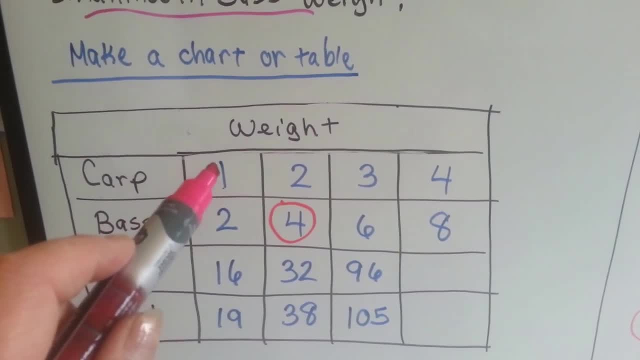 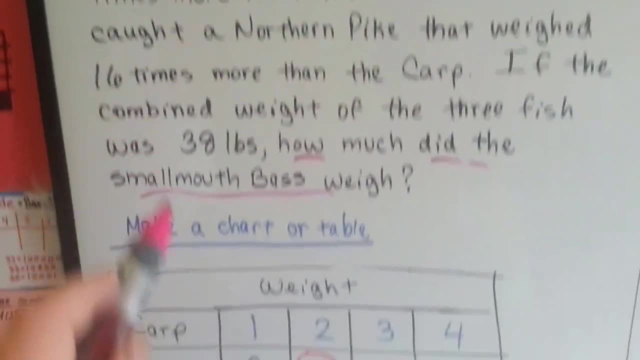 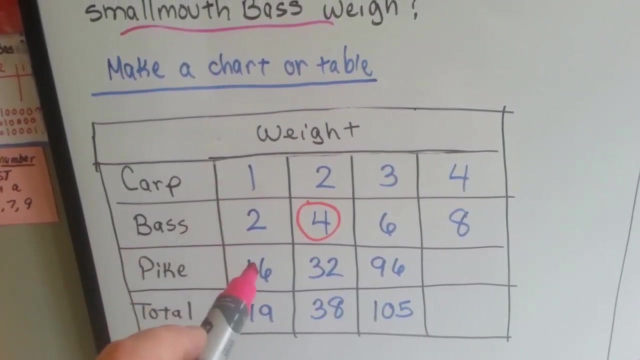 Now, if the carp weighed one pound, we know that the bass weighed two times more than it And the pike, it says, weighed 16 pounds. So it's 16 times more than the carp. So if the carp was one pound, then the bass would be two pounds and the pike would be 16 pounds, because 16 times one is 16.. 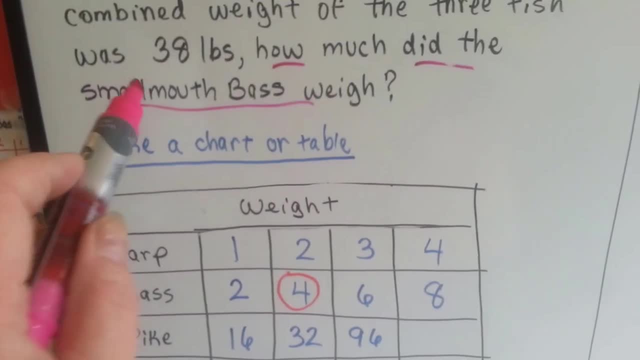 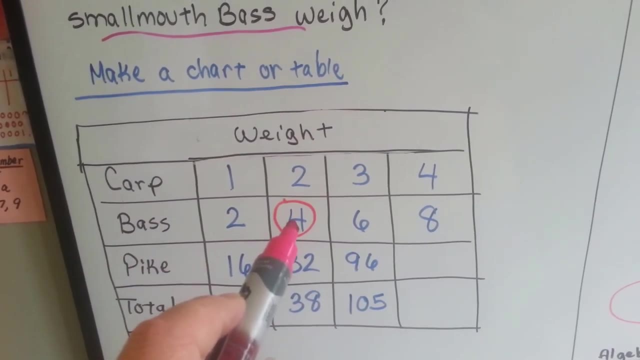 We total them together and we get 19.. Well, it says the total was 38, so you can already see the answer. If the carp weighed two pounds and the bass weighed two times more than it, then it would be four. 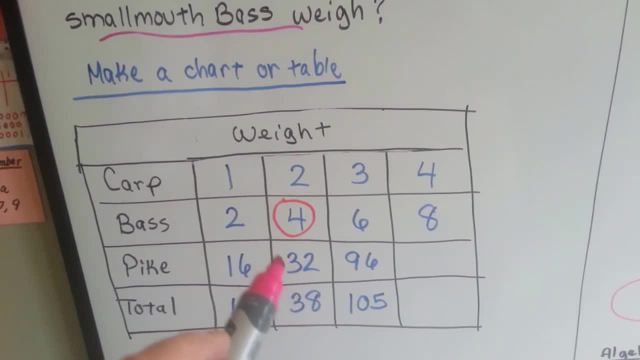 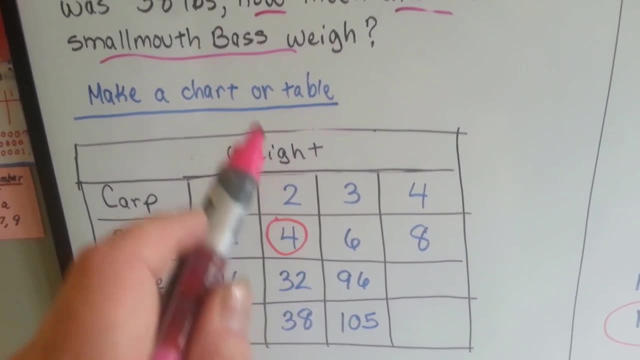 And if the pike weighed 16 times more than the carp, 16 times two is 32, when we add them up they're 38 pounds. That means the bass weighed four pounds. We know how much the bass weighed, see. 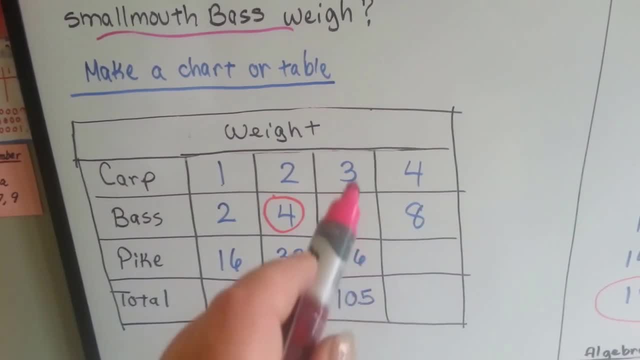 So making this chart or table really helped. We know that's too much, We know to not even finish the chart because that's going to be way too big, and we found our answer alright. So make a chart or table. 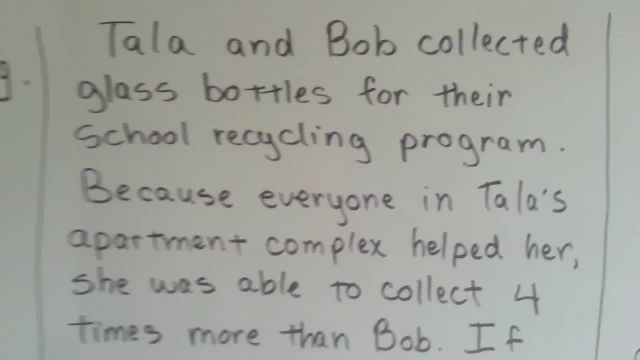 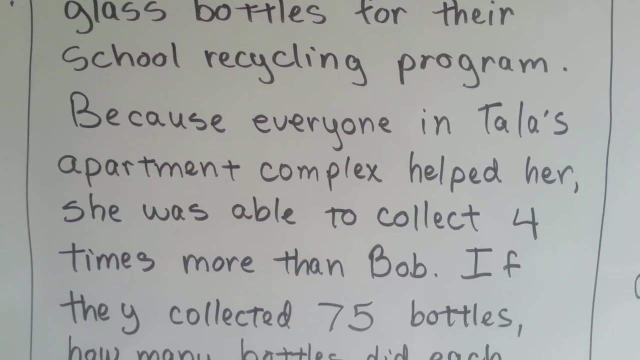 How about this one? Tala and Bob collected glass bottles for their school recycling program. Because everyone in Tala's apartment complex helped her, She was able to collect four times more than Bob Boy. was she lucky If they collected 75 bottles? 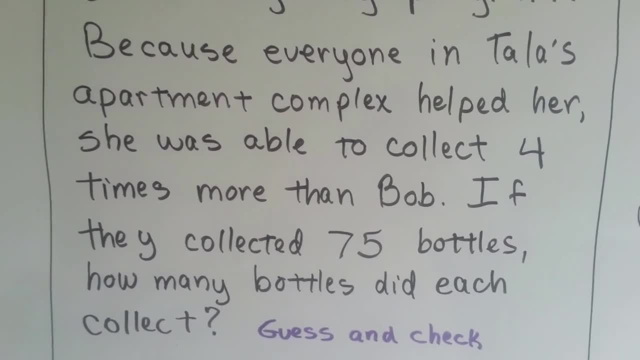 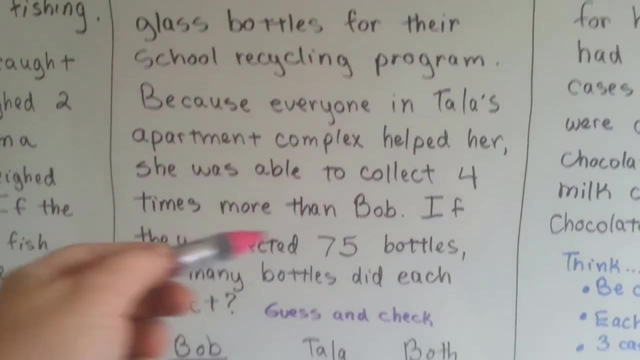 how many bottles did each collect? So we're going to guess and check. alright, So here's our information. Bob collected some amount. We don't know what. it is okay, It's just. N Tala collected four times more than Bob. 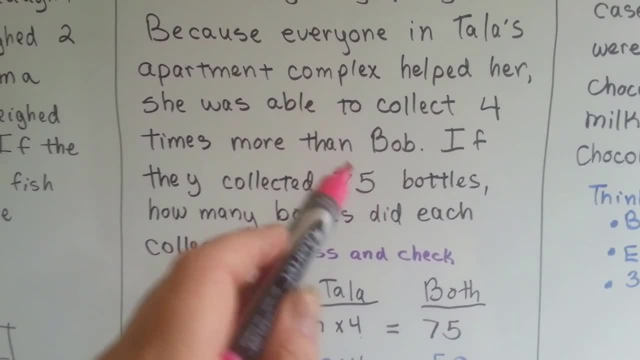 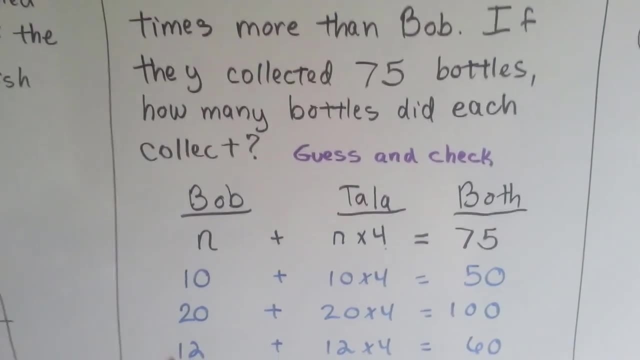 So it's four times more than that N, But together they collected 75.. Now we can actually use algebra to solve this, but I'm going to show you that at the end We're going to try, guess and check, okay. 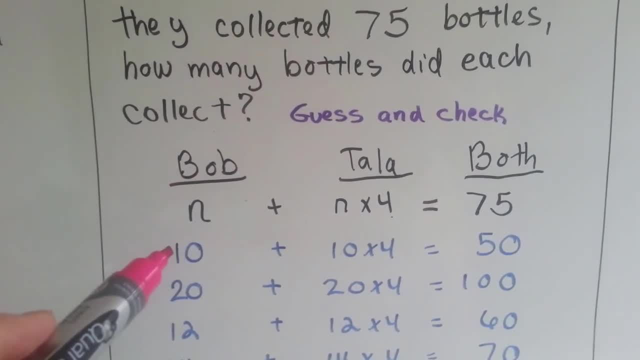 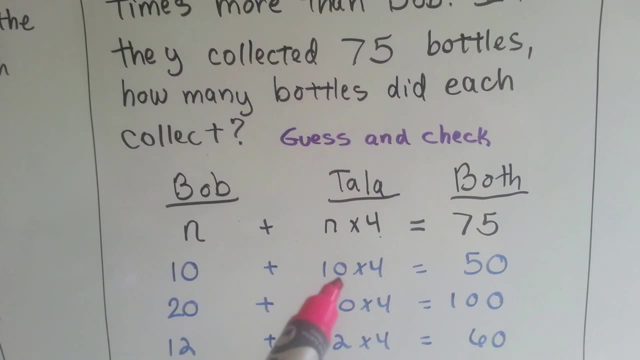 So let's just guess that Bob did 10,. alright? Well, if Emma did 4 times more than his 10,, that means she did 10 times 4. That's 40. Now we add his 10, and we get 50.. 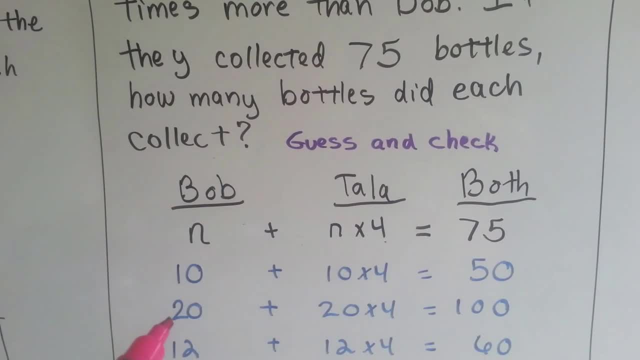 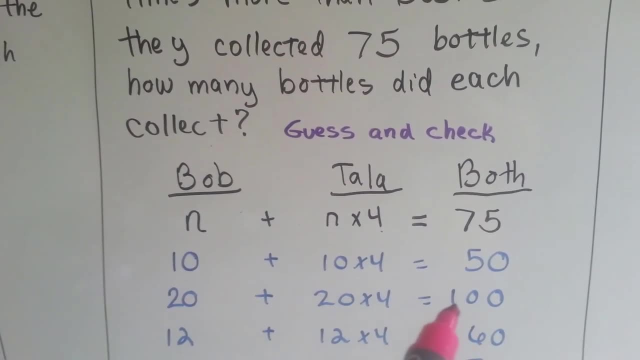 That's not enough. That's not 75.. So let's try 20.. If Bob collected 20, Tala collected 4 times 20.. That's 80.. 80 plus 20 is 100.. That's too big. 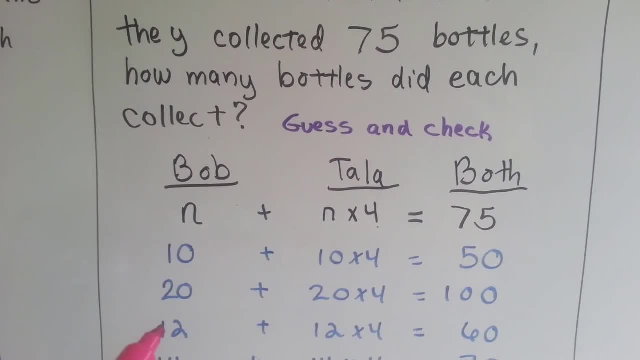 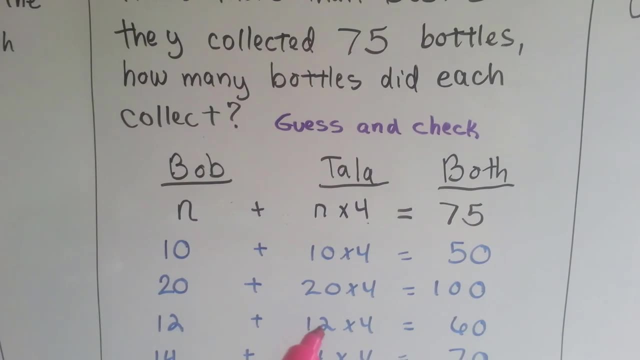 What if Bob did 12?? Let's go back down to a smaller number, because the 100 was too big. Well, that means Tala did 4 times 12.. Well, that's 48, and 48 plus 12 is 60.. 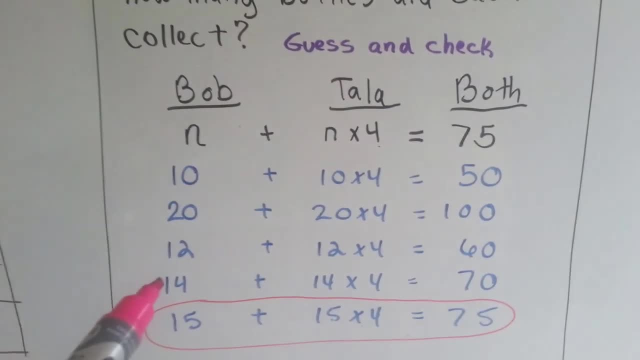 So that's not big enough. We've got to go back up again. So I tried 14, and that brought me to 70, and that wasn't enough, but it was close. so I went up by one more because we were so close. 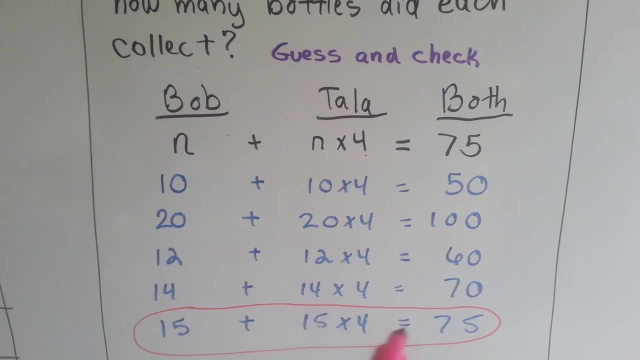 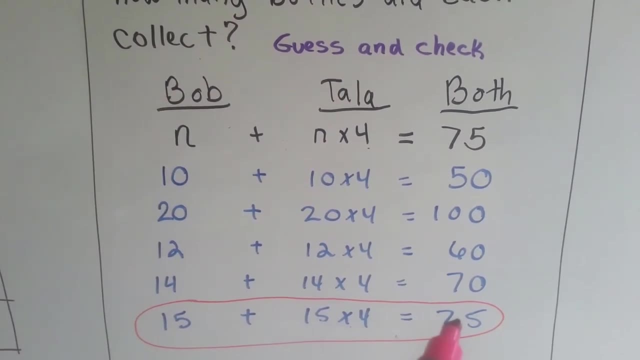 We were at 70. And then I found out that this worked. 15 worked, because 15 times 4 is 60, plus 15 that he collected would be 75. Now we could have done this a lot quicker with algebra. 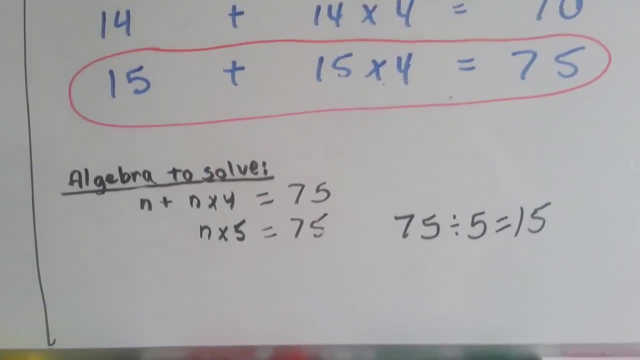 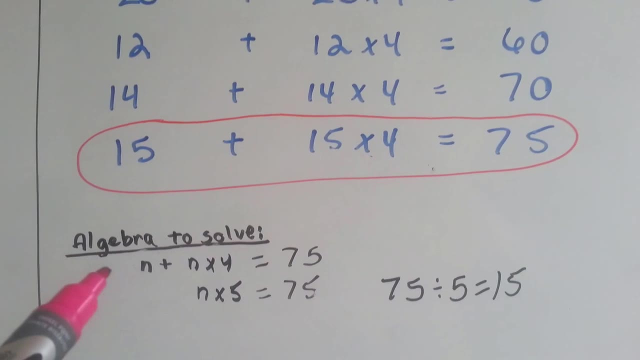 and I'm going to show you this really quick. and if you can't follow along, that's okay, because algebra is up there. It's a higher level of math. If you can follow along, then good for you. So we know that Bob collected n. 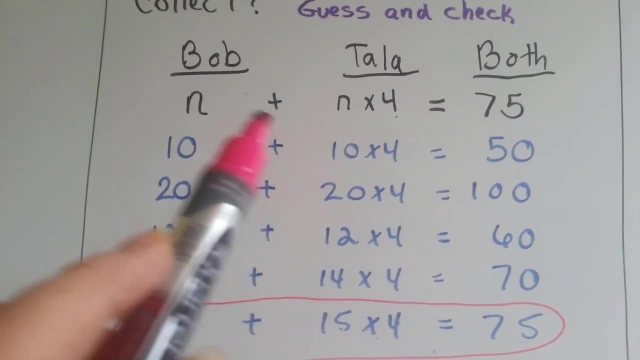 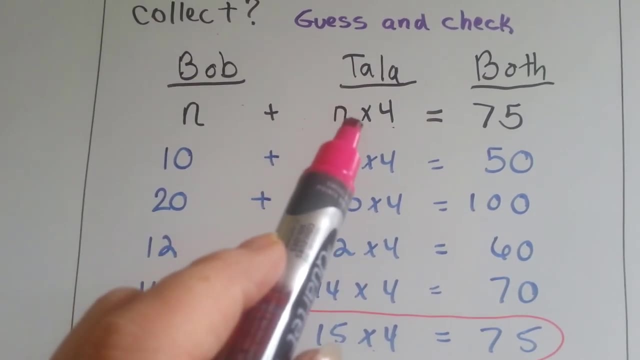 and Tala collected n times 4.. Well, that means that she had 4 n's right n times 4 means n plus n plus n plus n. Well, we could add his n onto that and get 5 n's, alright. 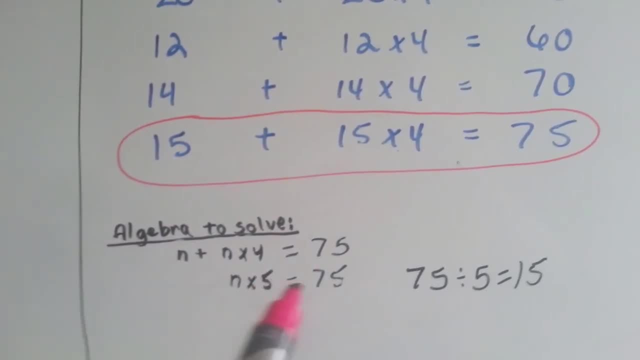 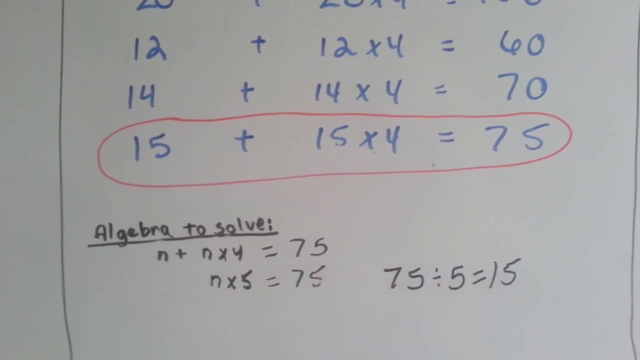 Which means 5 times n. Then all we have to do is say some number times 5 equals 75. Then we can do the inverse and divide by 5 and get 15, which is a lot quicker than guessing and checking, see. 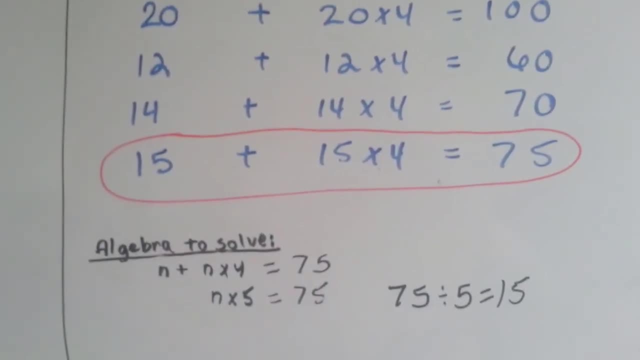 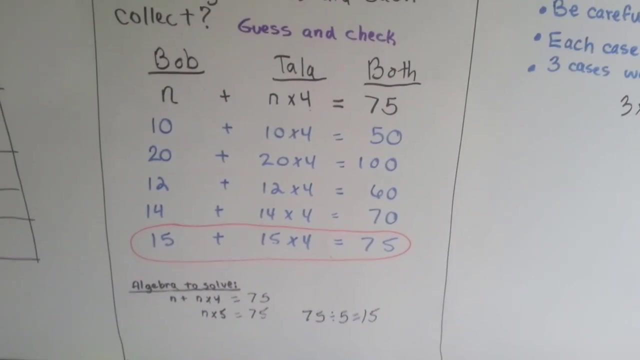 5 n equals 75.. 5 times n equals 75, see A lot quicker to do algebra. People say, oh, what do you use algebra for? in real life I would never use algebra And actually, if you know how to do algebra, 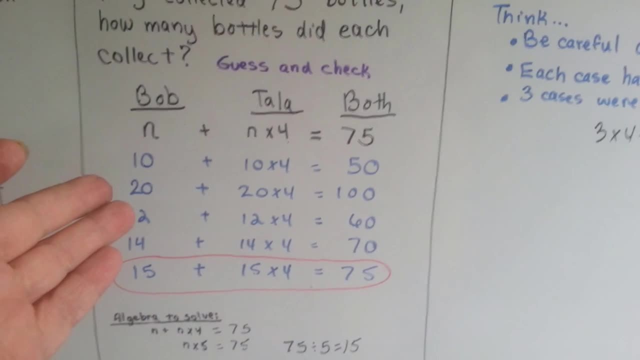 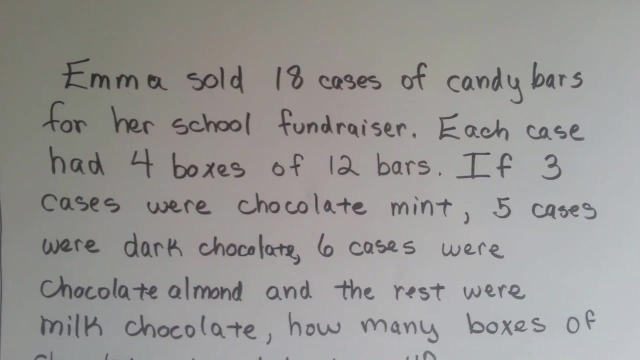 you'll see that it's a lot quicker than guessing and checking, okay, Okay, so let's look at our last one. Emma sold 18 cases of candy bars for her school fundraiser. Each case had 4 boxes of 12 bars. 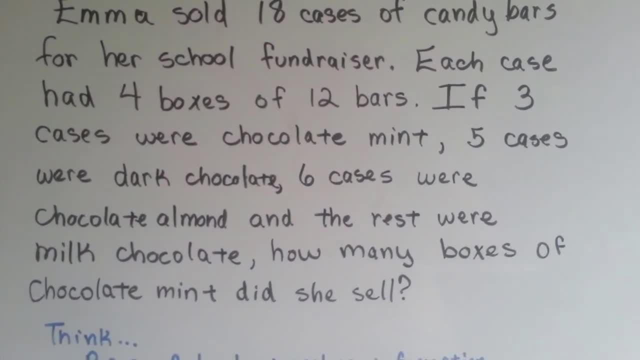 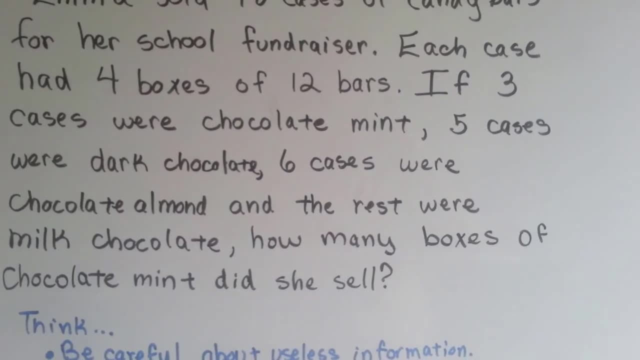 If 3 cases were chocolate mint, 5 cases were dark chocolate, 6 cases were chocolate almond and the rest were milk chocolate, how many boxes of chocolate mint did she sell? Okay, well, be careful about useless information. What is it asking us? 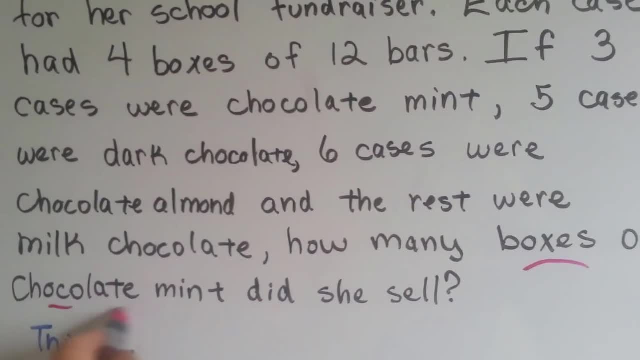 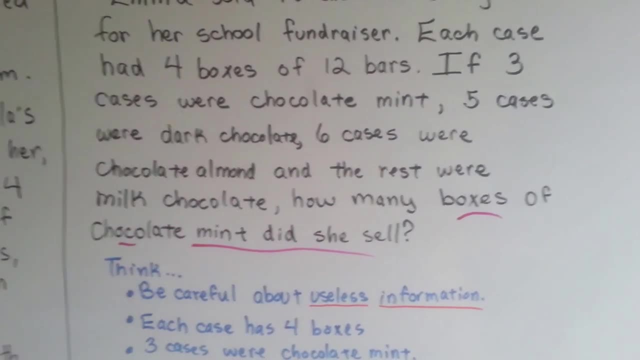 It's asking us: how many boxes of chocolate mint did she sell? So is it important? how many cases were dark chocolate or chocolate almond or milk chocolate? No, That was all useless information. The only thing that is important is the chocolate mint ones. 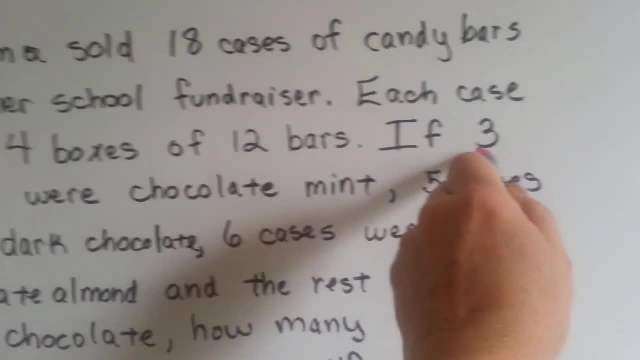 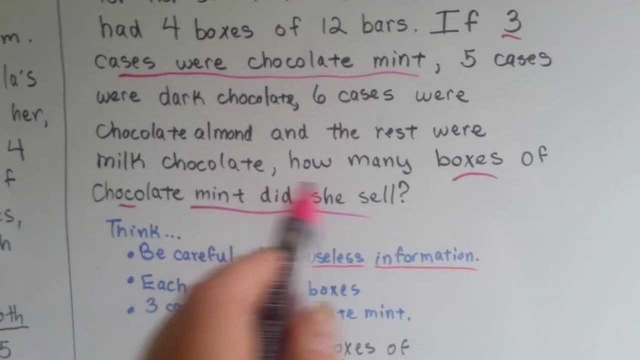 which is right here. She had 3 cases that were chocolate mint. That's the important information. Now, what else is it asking us? How many boxes Did she sell? Is it asking us, how many bars? So even the bars is useless information. 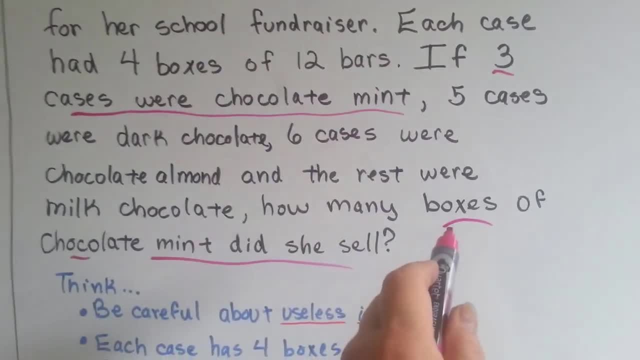 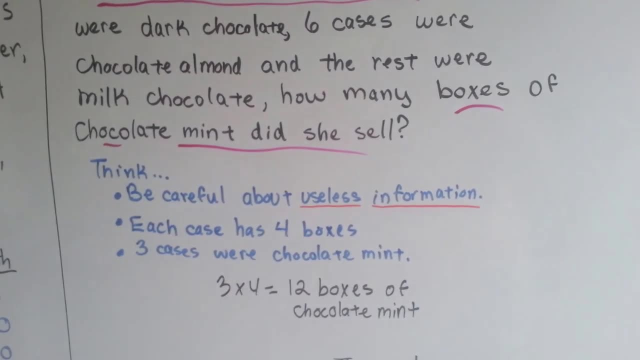 We don't need to know how many bars are in a box, because it's asking us how many boxes. Well, 3 cases. there's 4 boxes in each case, 3 times 4.. That was an easy one. She sold 12 boxes of chocolate mint.